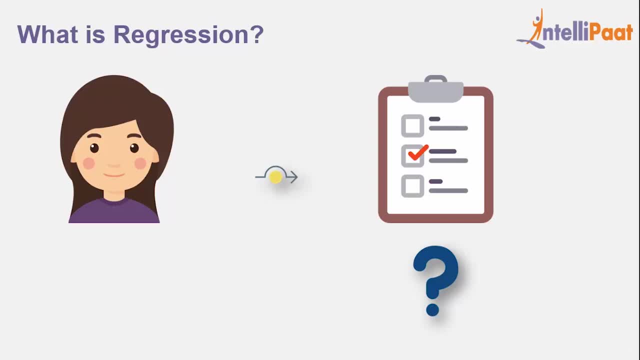 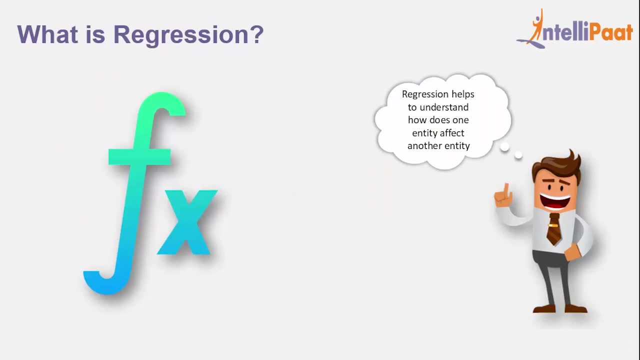 variable over here, and gender is the independent variable. So, in simple terms, regression helps you to understand the extent of relationship between two variables. So now that we've understood what exactly is regression, it's time to understand logistic regression. So logistic regression is a. 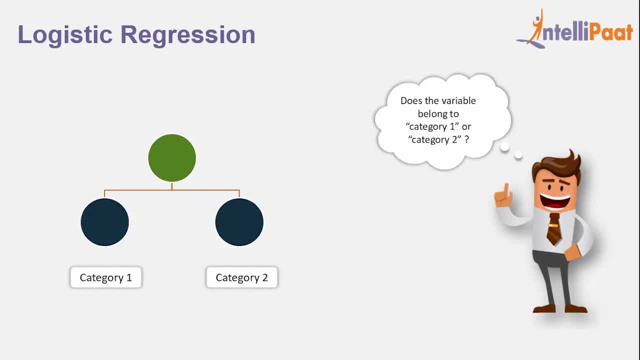 regression technique. where the dependent variable is categorical, We determine the probability of the observation belonging to a particular category. So let's look at an example to understand this better. Over here, we're trying to determine the probability of rain based on independent variables such as temperature and humidity, Or in other words, 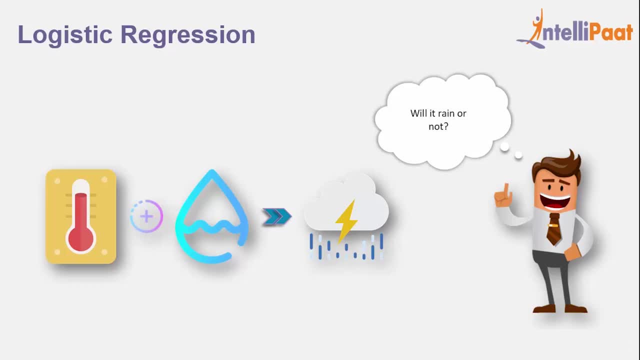 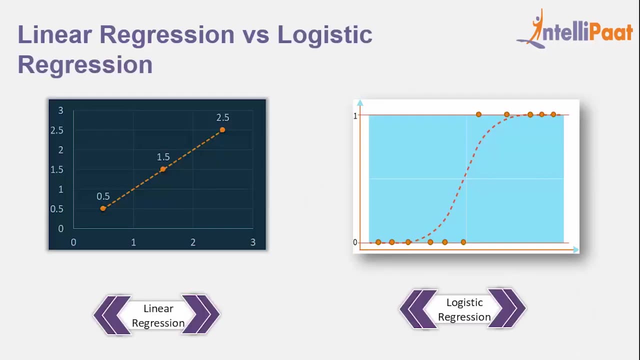 we're choosing a category, namely yes or no, for the question: will it rain? So this is logistic regression for you Right now. we'll head on and understand the difference between logistic regression and linear regression. In linear regression we fit a straight line, That is, for a given value of x. there, definitely, 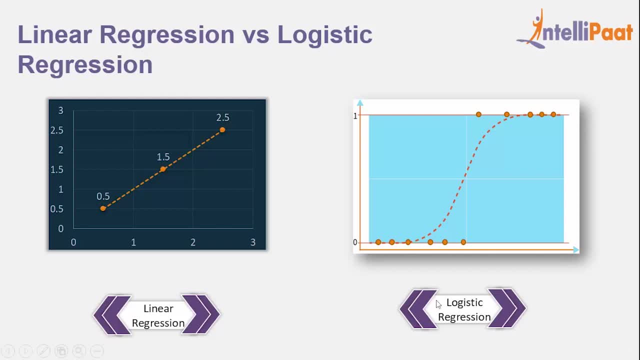 exists a y value which falls on the line. Or in other terms, we can say that there is a linear relationship between the y variable and the x variable. So you can take the example of an employee's salary and age. So let's say the x-axis denotes the employee's age and y-axis denotes the. 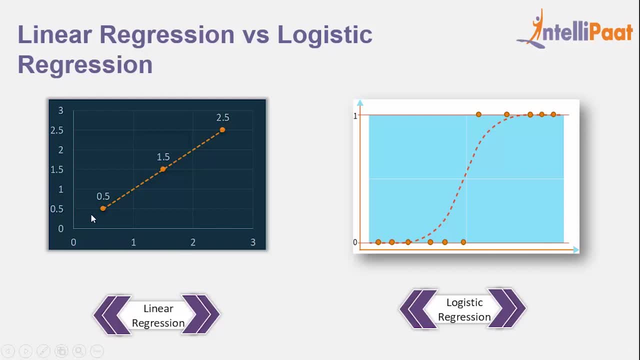 employee's salary. So as the employee's age increases, the employee's salary increases. The employee's salary would also increase linearly. So this is linear regression. But what happens in logistic regression is: the dependent variable is categorical And hence the dependent variable. 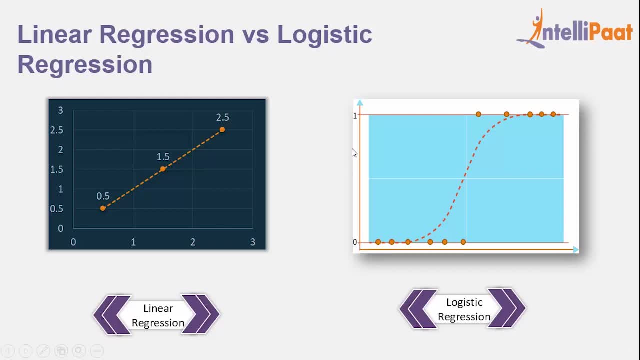 can only have two values, that is, either 0 or 1.. Now let's understand this better. So let's say over here: the x-axis denotes the number of runs scored by Virat Kohli and the y-axis denotes whether Team India has won the match or not. Let's say: this line over here denotes the number of runs. 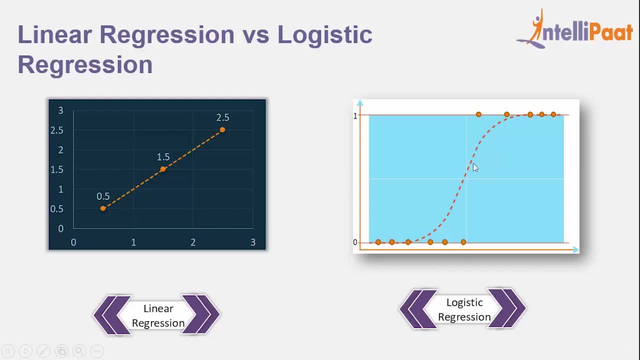 scored by Virat Kohli, and the y-axis denotes the number of runs scored by Team India. So let's say, over here, the x-axis denotes the number of runs scored by Team India, And hence the dependent variable is called the 50.. So what we can see from this graph is if Virat Kohli scores more than 50. 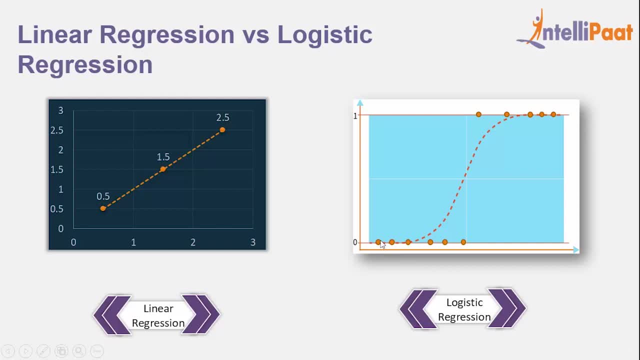 runs in a match, then there is greater probability for Team India to win the match. And if Virat Kohli scores less than 50 runs in the match, then there is a good probability that India might lose the match. Let's actually take these two points over here. So let's say this is around 50 runs or 49. 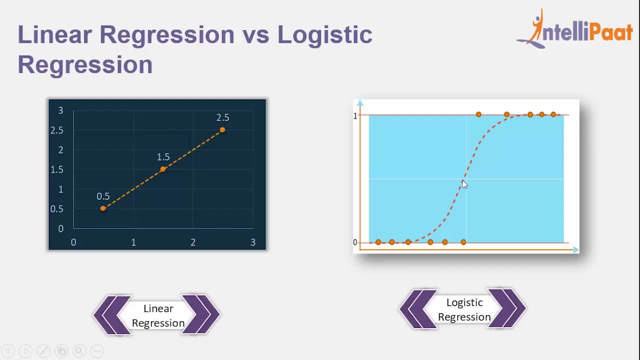 runs, the match would also be around 48% or 50%. Now let's take this. So let's say this is around 60 odd runs. So let's say, if Virat Kohli scores 60 runs, then the probability of India winning. 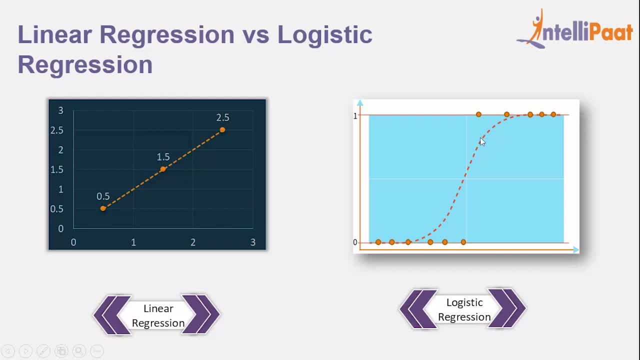 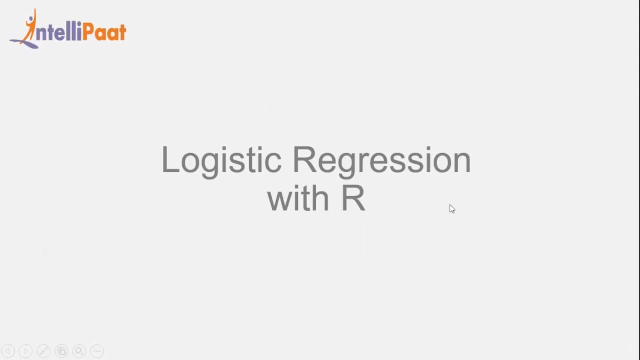 the match would be around 70% or 75% Right. So in linear regression we have a straight fit line and in logistic regression we have an S curve. So this S curve gives us the probability of the result being true or false. So it's finally time to implement the concept of logistic regression. 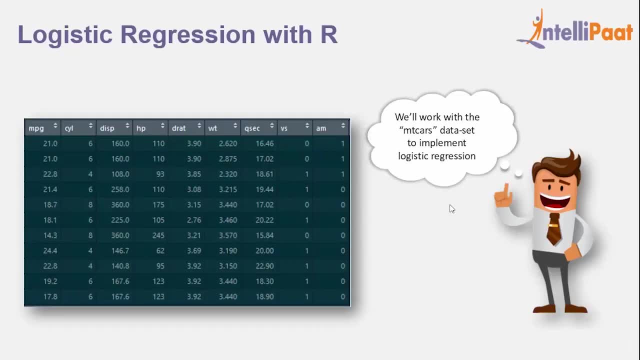 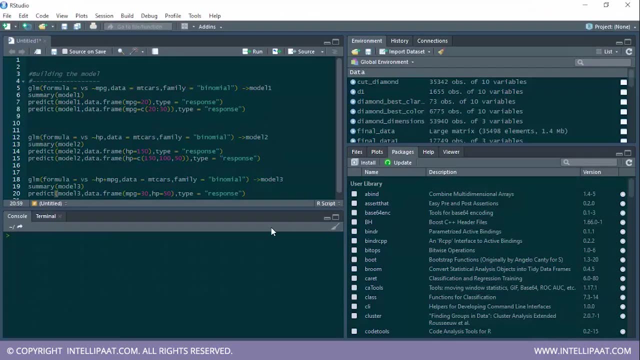 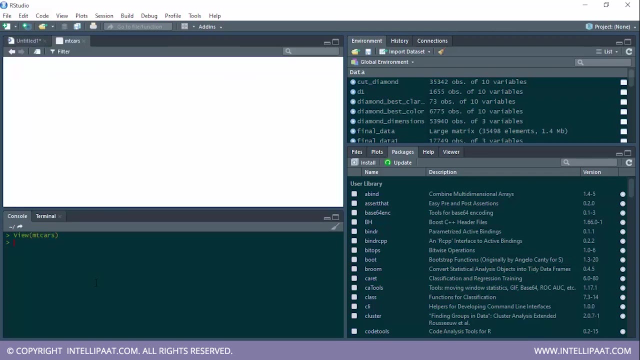 with R. So let's go ahead and do that. So we'll be working with the empty cars dataset to implement logistic regression. So let's head to R studio, Right? So this is how R studio looks like. So let's have a glance at the empty car dataset first. So I'll say: view of empty cars, Right? 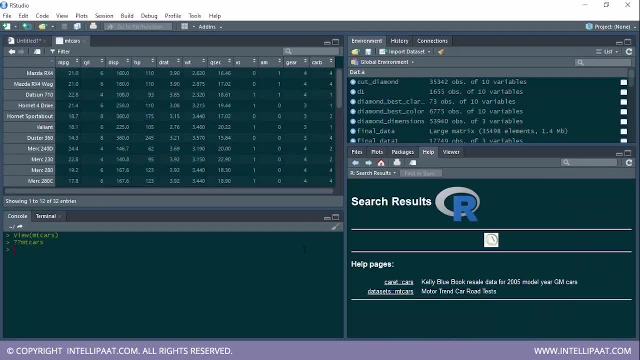 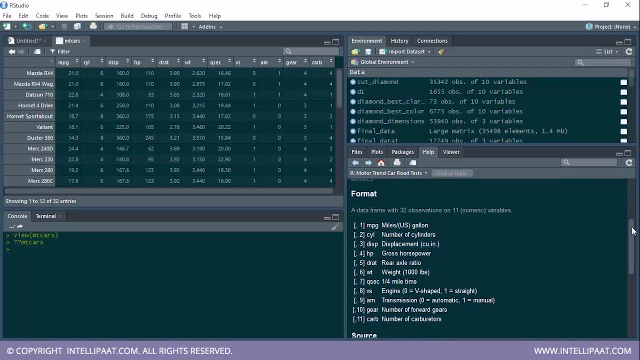 This is our dataset. Now let's understand this properly. So this is our dataset, which has 32 observations, or, in other words, we have 32 cars and these are the variables. So MPG is the miles per gallon, Sil is the number of cylinders in car. This is: 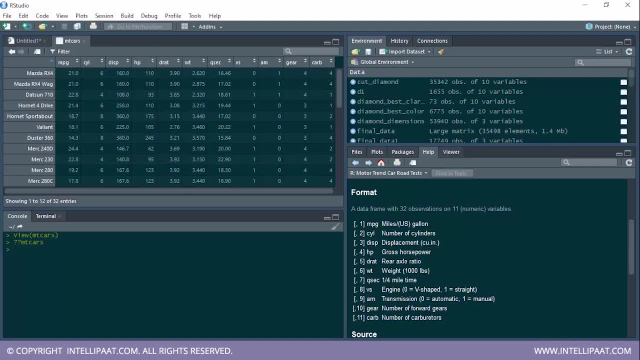 displacement, Then we have horsepower, Then we have rear axle ratio, the weight of the car, QSEC, VS being whether the engine is V shaped or straight, AM is for the transmission of the car, Gear is number of forward gears and carb is number of cooperators. 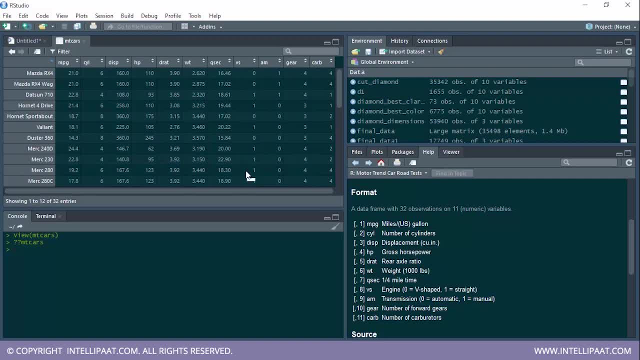 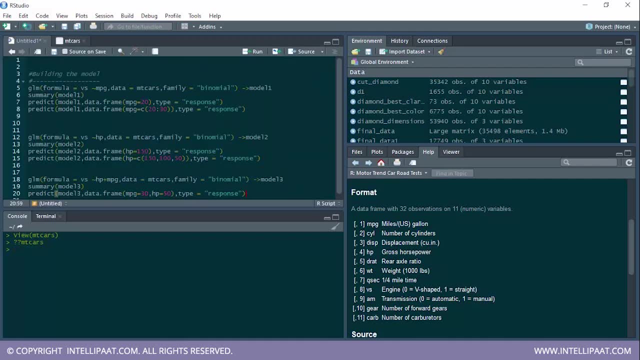 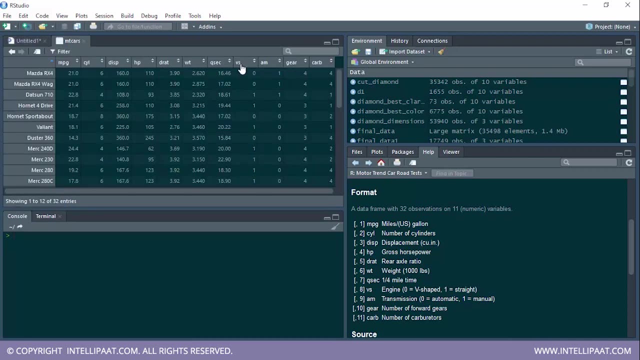 So in this example, we would try to determine whether the car has a V-shaped engine or a straight engine based on other variables. So let's go ahead and do that. So in the first case, I would want to determine whether the car has V-shaped engine or straight engine with respect to the mileage of the. 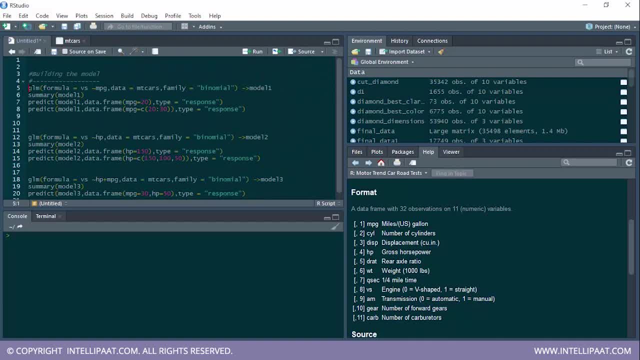 car. So let's go ahead and do that. We will be using the GLM function. So over here, the GLM function takes in three parameters. First is the formula. So over here, in the formula we have stated VS, tilde, MPG. that is, VS is our. 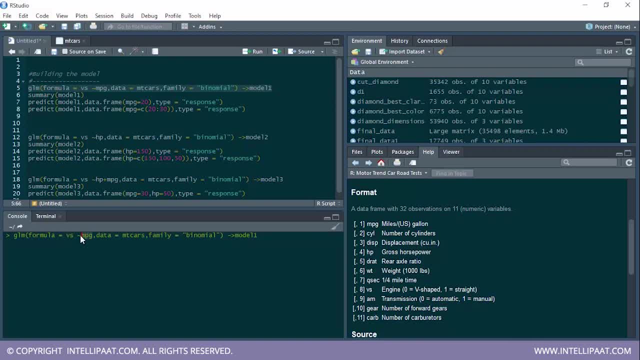 dependent variable and MPG is our independent variable. So whatever variable is given on the left side of the tilde symbol would be our dependent variable and whatever variables are given on the right side of the tilde symbol would be our dependent variable. So we have 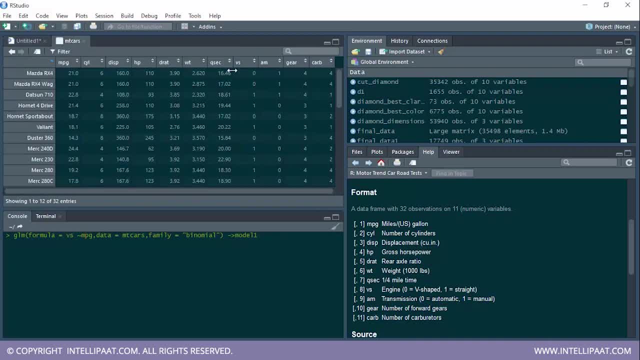 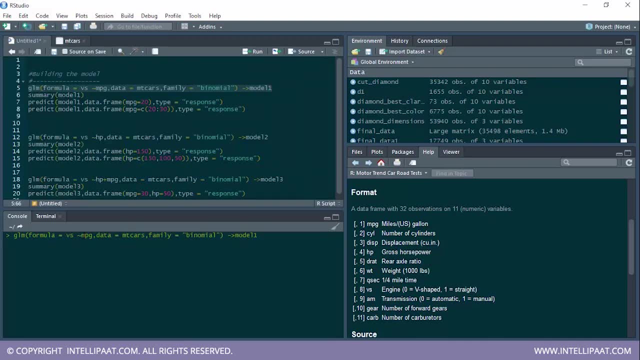 the independent variables. So we are trying to determine the type of engine of the car with respect to the miles per gallon of the car, Right? So this was our first parameter. The next is obviously the data set which we are going to give. So the data set is empty cars And the 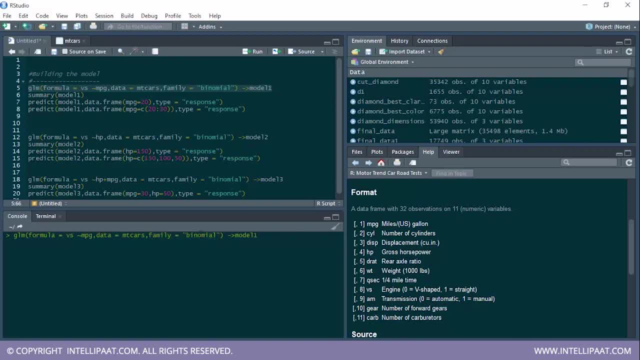 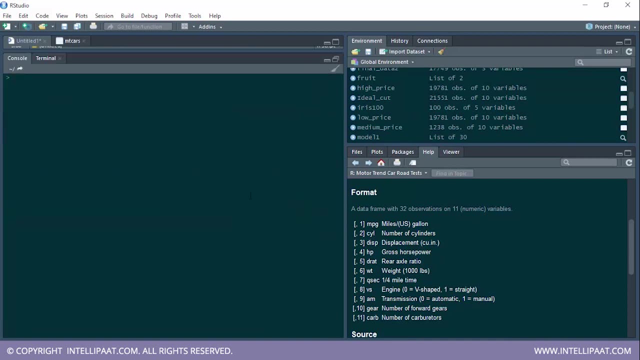 third parameter is the type of regression technique. So the type of regression technique used over here is binomial, That is, we are going to have just two values, either zero or one, And we'll store that in the model one. So we have successfully built a model. Now let's analyze this model and 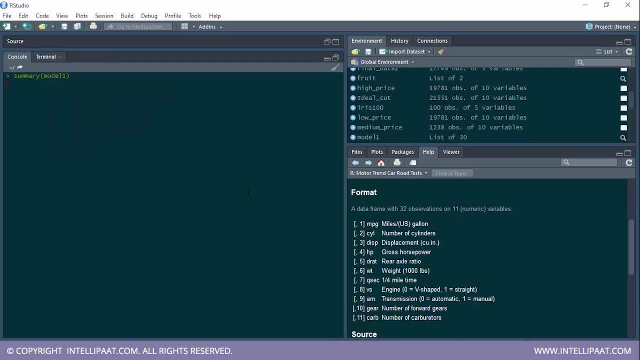 analyze this model. I'll say summary of model one. So this was the model which we build And we have some values over here, So let's understand these values properly. So I'll start with these three values over here. So we have null deviance, residual deviance and AIC. So what is null deviance? So in 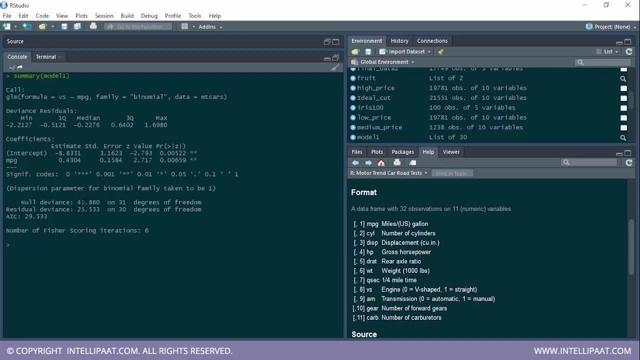 the model. null deviance gives up the accuracy of the model when the independent variable is just the intercept. Or in other words, we are trying to determine whether the car has V-shaped engine or S-shaped engine without any variables or without any independent variables. So when we're not, 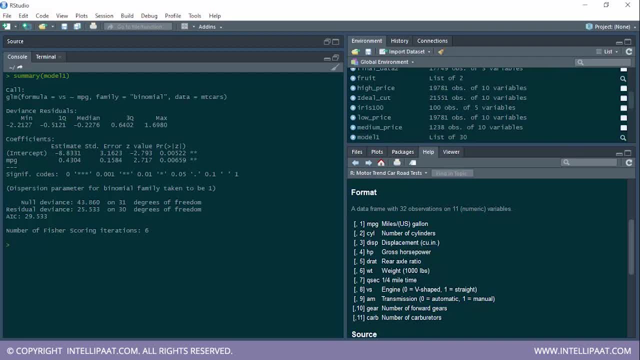 including any independent variables, then the deviance is 43. Now it needs to be kept in mind that any deviance or any sort of deviance should be as less as possible. Now, when we include this one variable in the formula, then we get the residual deviance. So when we include mpg into the 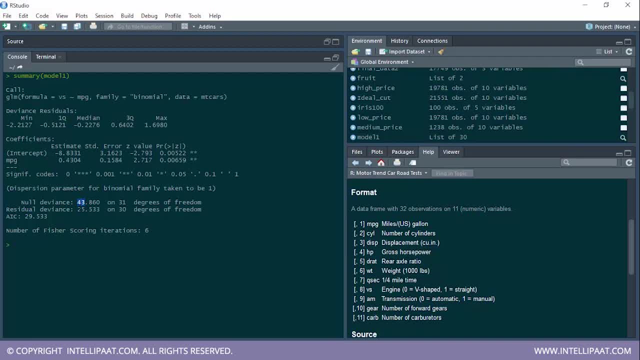 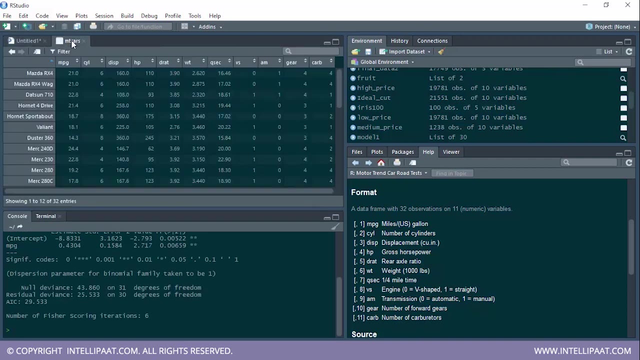 formula. then we see that the deviance has decreased from 43 to 25. And we also see that the degrees of freedom have decreased from 31 to 30. So decrease of freedom is nothing but the number of observations minus one. So the number of observations in empty cars data set were 32.. That is the number of degrees of. 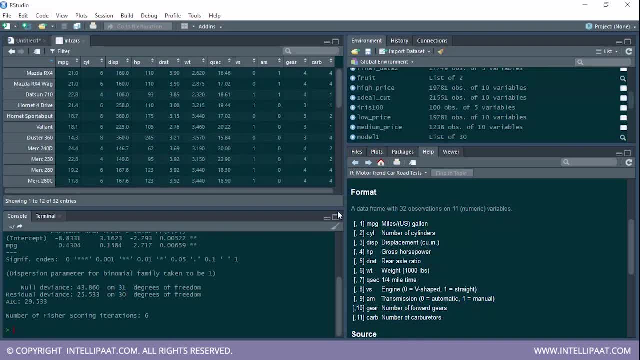 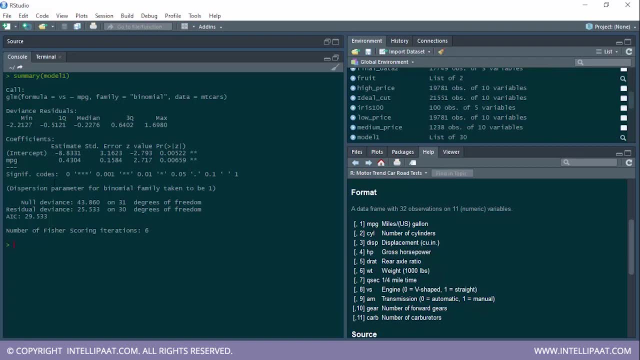 freedom is 31.. Now when we include another variable over here, the decrease of freedom reduces by one again and we get it to be 30. So basically, the point that I'm trying to see over here is initially the null deviance, that is, when we're not including any variable, then the null deviance is 43. When 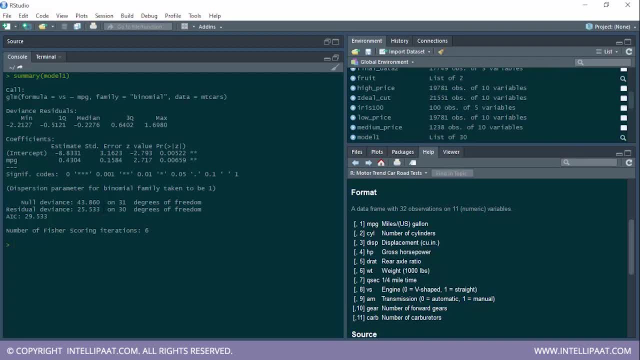 we include the variable mpg into this formula, then the residual deviance decreases. So when we and we get the residual deviants to be 25.. So this is null deviants and residual deviants, Then next we have AIC. So AIC basically stands for Achaic Information. 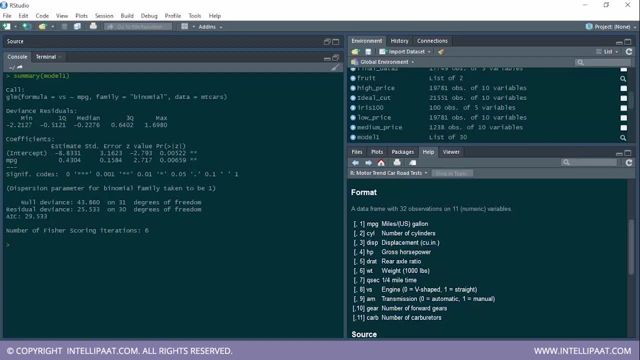 Criteria. Now this is helpful when we are comparing two to three models with respect to each other. So, in simple terms, basically, the lower the value of AIC, the better the model, Right. so these were the three values. now let's actually understand these values over here. So this over here which you see, so mpg then 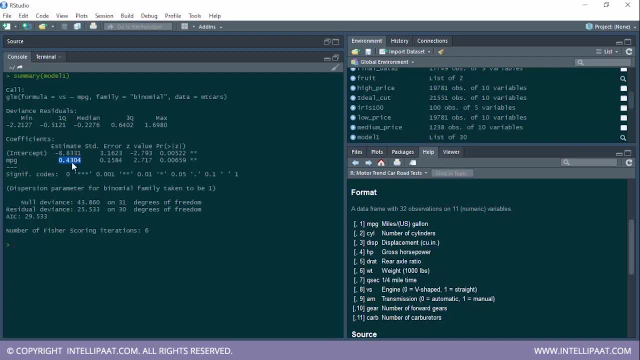 the estimate is 0.4304. that is, with every one unit change in the miles per gallon value we have, we see 0.43 units of change in the logit value of VS, Since because it's logistic regression. so we see that with every one unit. 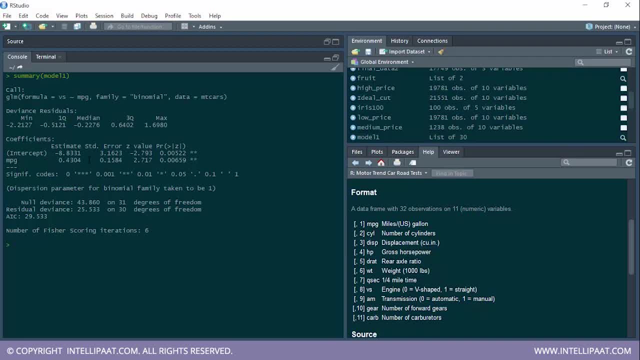 change. there is 0.3 units of change in the logit value of VS. Now, this is the most important value over here, the p-value. so with the help of p-value, we try to determine whether this variable is significant or not. So these quote which you see over here. So if we 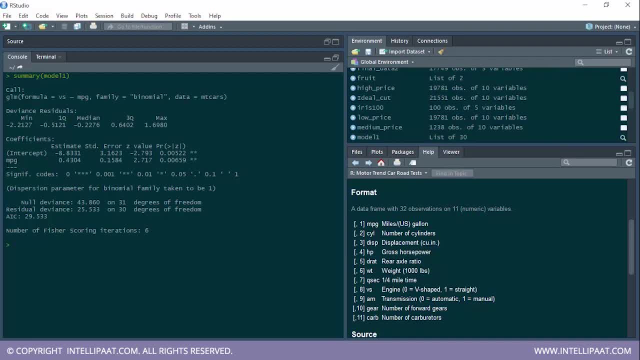 just have one dot over here, then that would mean that the variable is 95% significant. if we have one star, then that would mean that that is 95% significant. If we have two stars, then it would mean that the variable is 99% significant. and if we 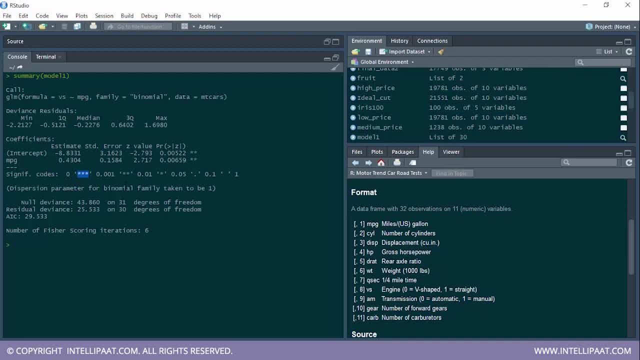 have three stars, then it would mean that the variable is 99.99% significant, right. And since we see that MPG has two stars over here, then it is significant with a confidence interval of 99% right. So we have built the model over here. 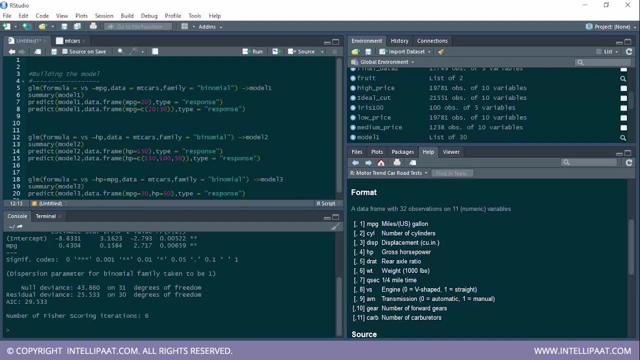 Now it's time to check the accuracy of the model. So what we'll do is we'll predict this on some other dataset, So let's go ahead and predict these values. So now, to predict the values on some other dataset, we'll be using the predict function. 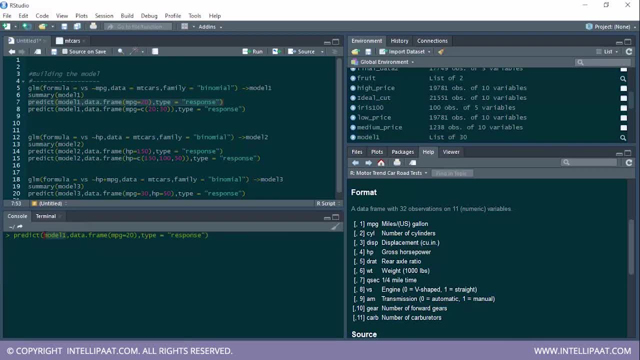 This again takes three parameters. So the first parameter is the model which you built. Next takes in the independent variables. So over here, since the independent variable which we had was MPG. So we'll take this MPG and create a data frame out of it which will just comprise: 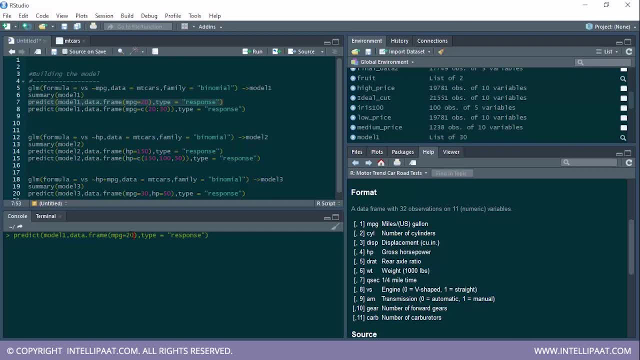 of one row, That is, we are trying to determine whether the car will have V-type engine or S-type engine with respect to the MPG when it is 20.. And we'll say: type is equal to response, because we need the probability of it, right. 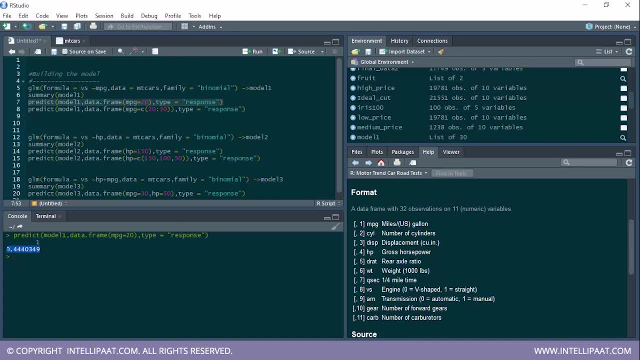 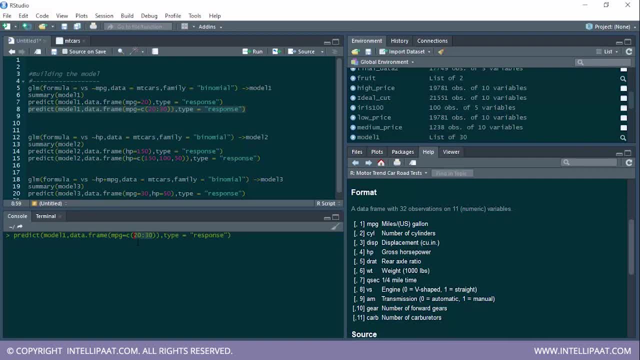 That is, the miles per gallon value would start from 20 and then we'll go like 21,, 22,, 23 to 30. Now let me determine what would be the probability of the engine being V-type with respect to these values. 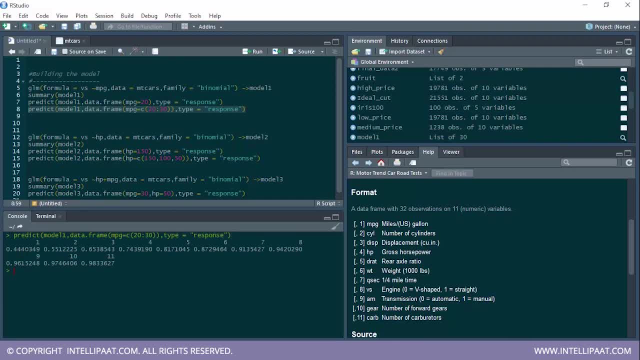 Right. So what we see over here is, as the MPG value increases from 20 to 30, we also see that the probability of the engine being V type increases. so the probability is increasing from 44% to 98%, and this is. 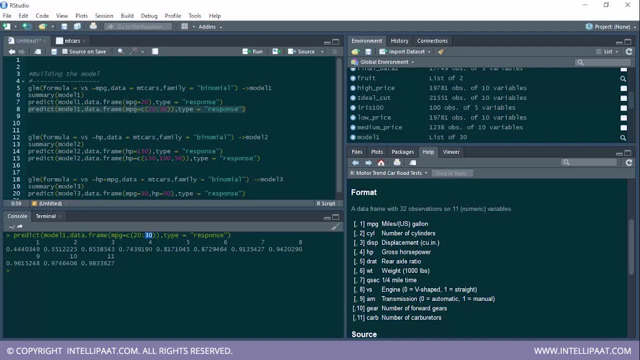 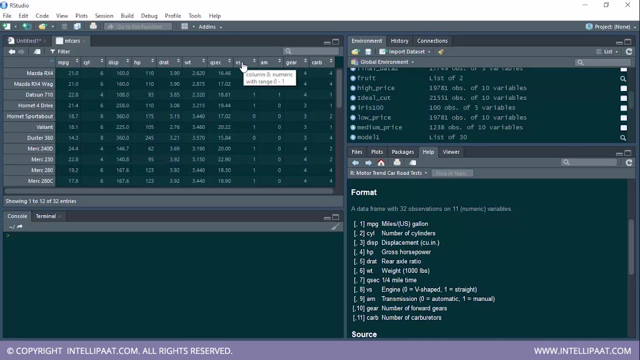 the maximum over here. so when the miles per gallon value is 30, then there is 98% probability that the engine is of V type. now, instead of miles per gallon, let me take another column to determine whether the engine is of V type or S type. so now 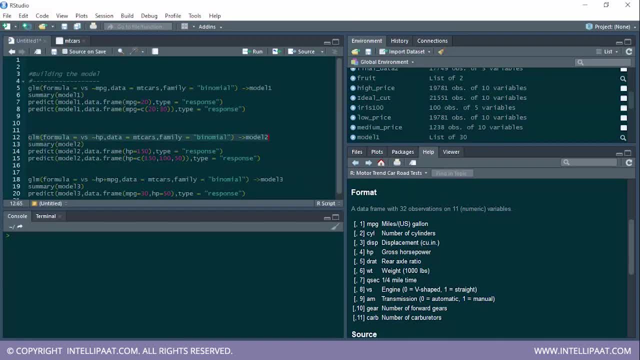 I'll be taking the HP column, so this time the formula will be VS. tilde symbol: HP. that is, the dependent variable is VS and the independent variable is HP, or in other terms, I'm trying to determine whether the engine type is V or S with respect to the 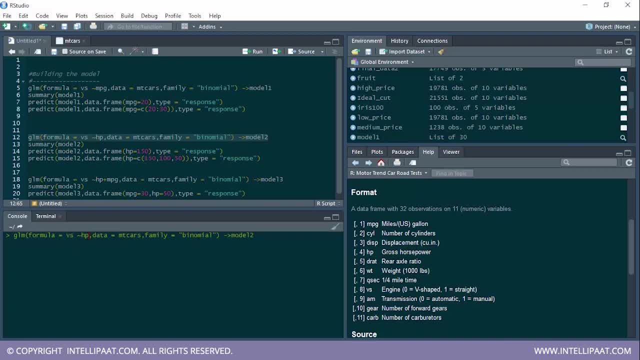 horsepower of the car. again, the data used is empty cars and family vehicles or other vehicles and so on and so forth. so this will be the is binomial, because I want a logistic regression for this, so I'll store this in model 2. now let me compare the summary of model 1 and model 2 and let 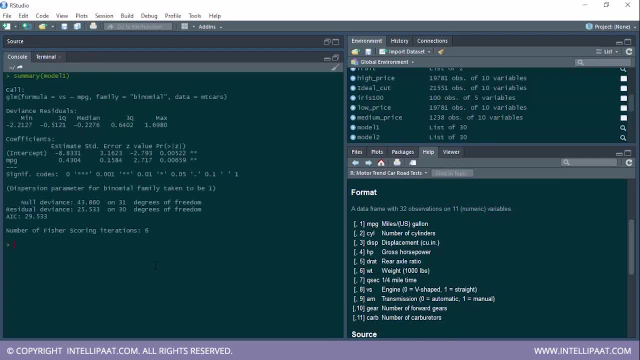 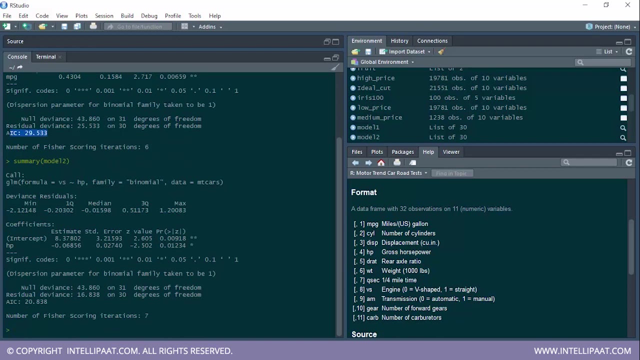 me determine it properly. so model 1 and similarly, summary of model 2, right? so let me first start off by comparing the AIC values of these two. so AIC value of model 1 is 29 and AIC value of model 2 is 20. that, a second model, is much. 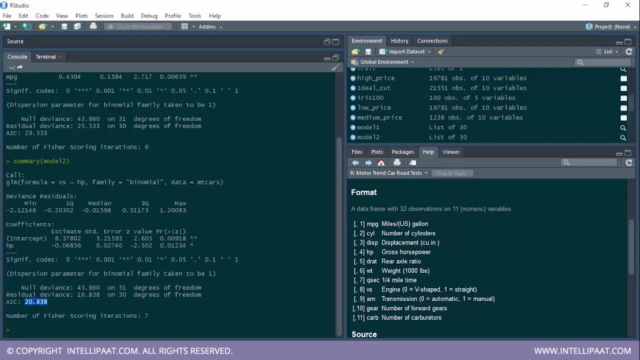 better and significantly better than model 1 because the AIC value reduces by almost 9 units and similarly, if we look at the null deviants over here, so null deviants is same. that is when we are not including any variable in the formula, but when we go ahead and include the variable. so over here in the model 1 we 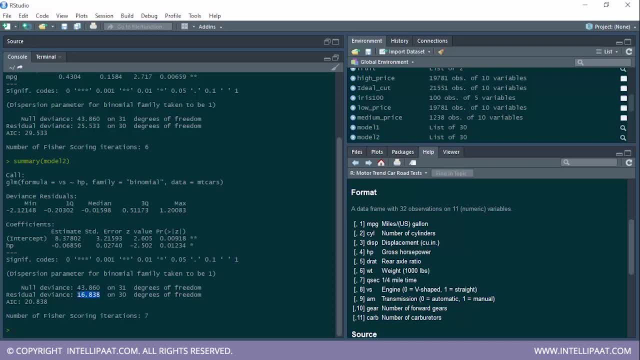 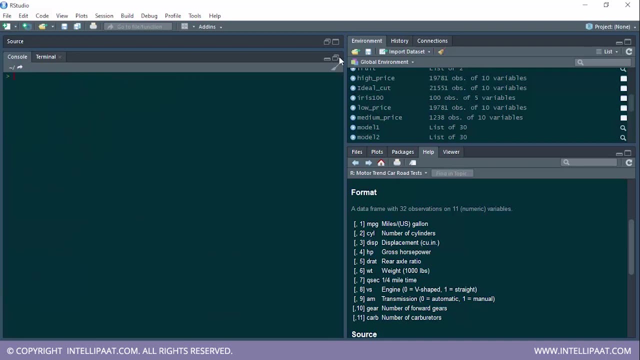 included MPG and in model 2 we included HP. so when we included horsepower, there is a greater reduction in residual deviant, or in other terms, we can see that HP is more significant than miles per gallon, right? so again, let us go ahead and predict some values with respect to horsepower. 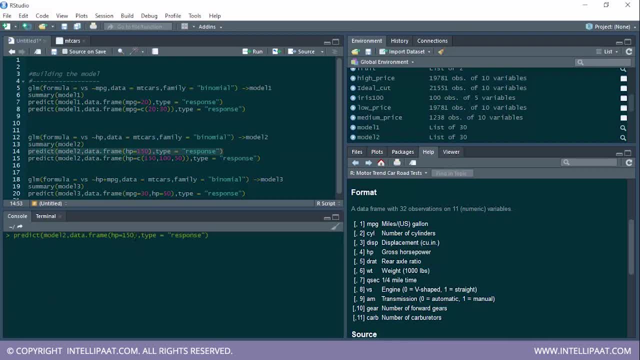 right now I'd want to determine whether the engine is V type or S type when the horsepower is 1.5. So you see, the model model 1 has a stock V type which is 50 units. so again, three parameters: first is the model which we build, which is model 2. next is: 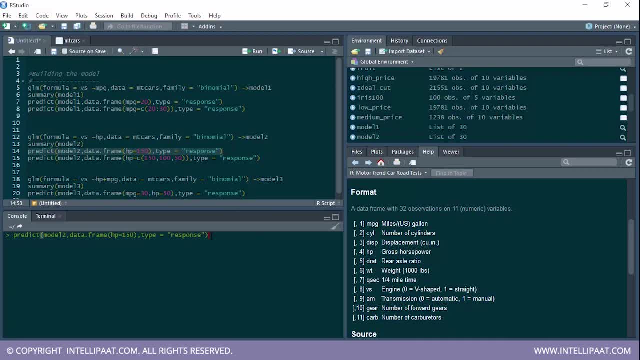 the data frame or the set of input values, and we are just giving one h top value over here. type is response, because we would need the probability right. so the probability of the engine being V type is just 12 percent. now. this is quite low. so what we will do is we will give a set type as well. 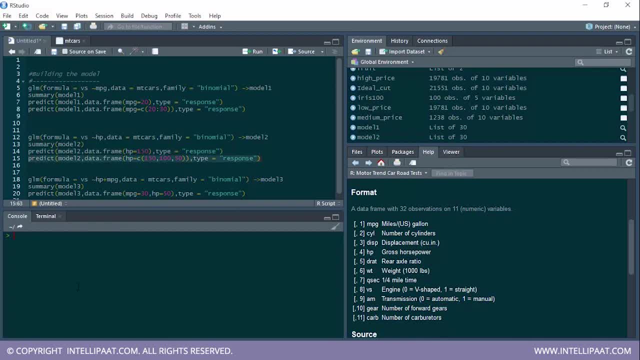 of values now and determine how does horsepower affect the type of engine. So this time I am giving three values for horsepower. The first value is 150, second value is 100, third value is 50. So what we see is, as horsepower decreases, there is a greater probability for the engine. 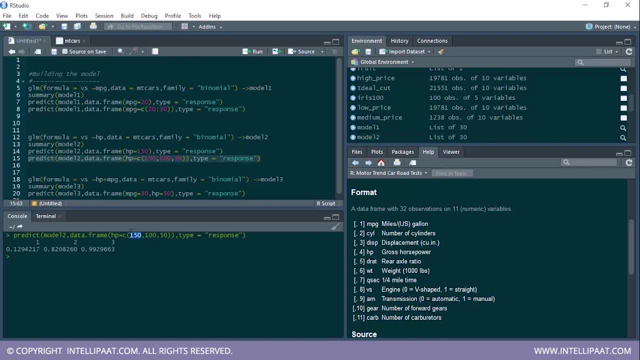 to be of V type. So, over here, if horsepower is 150, then most probably this type of car has a straight engine, and if the horsepower is 50 units, then most probably this type of car has a V type engine, Right? so this is how we determine whether the engine has, whether the engine is V type or S. 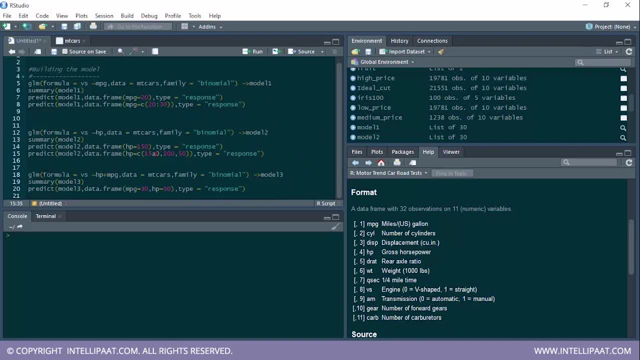 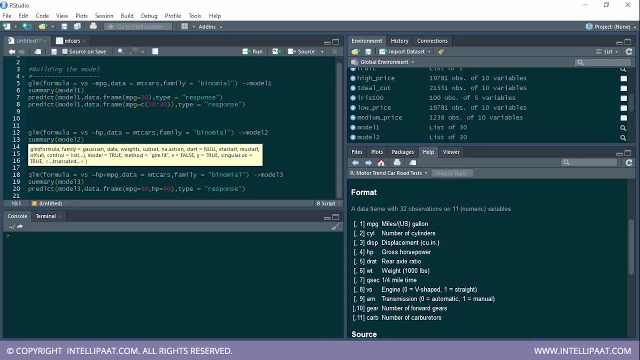 the horsepower and MPG into the same formula and see what happens. So this is my third model over here, where the formula over here is this: So again, VS is the dependent variable and HP and MPG are the independent variables. That is, I want to determine how would these two variables combined? 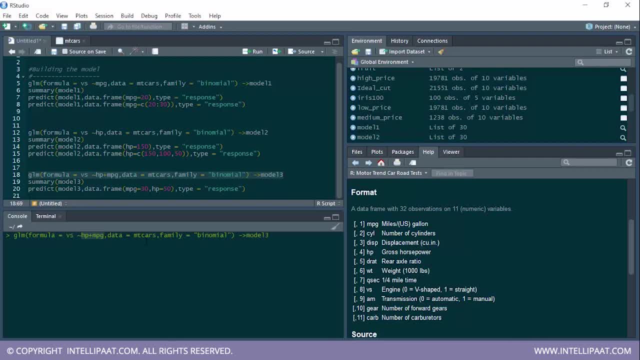 would affect the type of engine used in the car And again, data is empty. cars and family is binomial. So I'm going to include the V type engine and MPG into the same formula and see what? because I'm building a logistic regression model and I'll store this in. 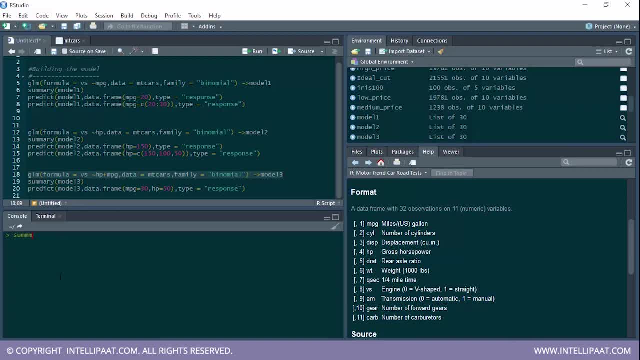 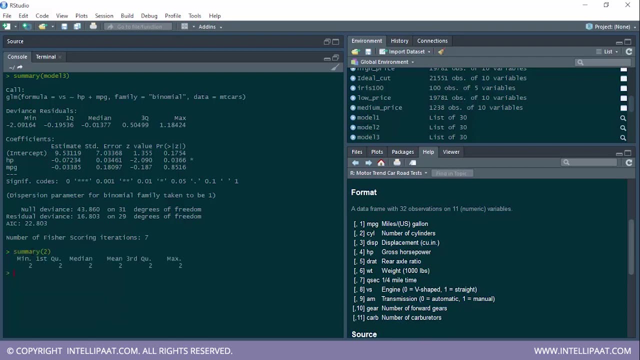 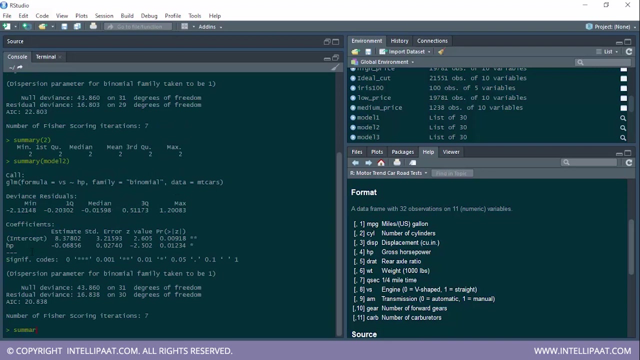 model 3 right now. well, let me check out the summary of this model as well. so I'll say summary of model 3 and let me have a look at this. summary 3, summary 2, right summary of model 2, and next we have summary of model 1. so let 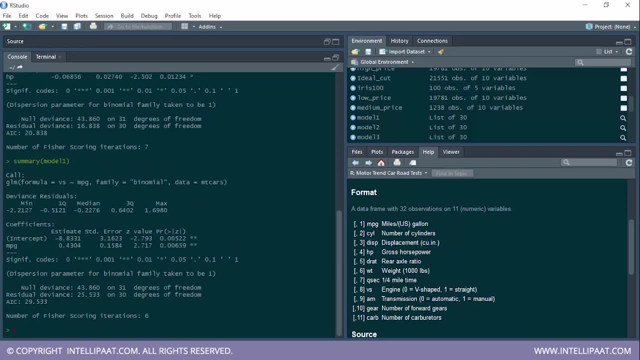 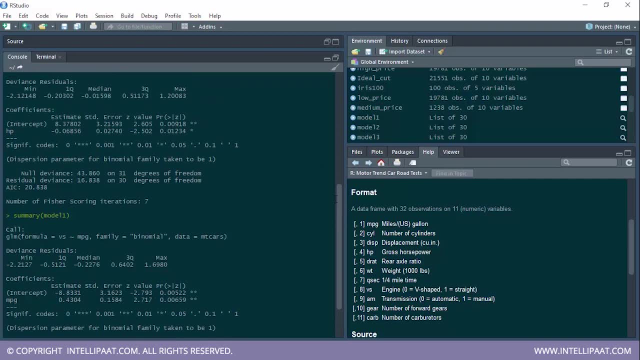 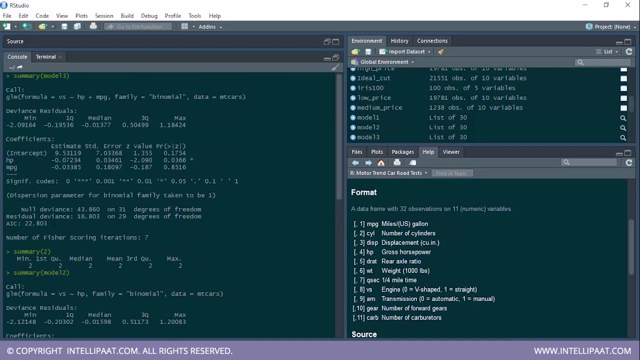 me start off by checking the Fisher score. let me start off by checking the AIC values over here. so for model 1, AIC value is 29. for model 2, AIC value is 20 and for model 3, which is over here, the AIC value is 22. so what we see is AIC value as the best. 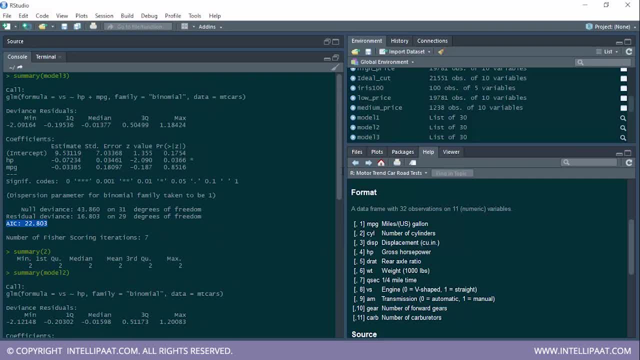 for the model 2. now let's understand the model 3 properly over here. so what we see is when we include HP and MPG both of them in the same formula, now just HP is the only variable which is significant and MPG, or miles per gallon, is not adding any value to the value of the model 2. model 3 is the only variable. 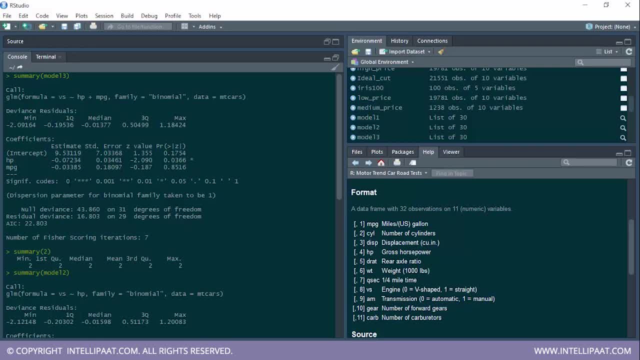 which is significant, and MPG, or miles per gallon, is not adding any value to the model and that is why, when we compare model 3 and model 2, if we just include HP, that is a much better model. so including MPG into the model, which HP is. 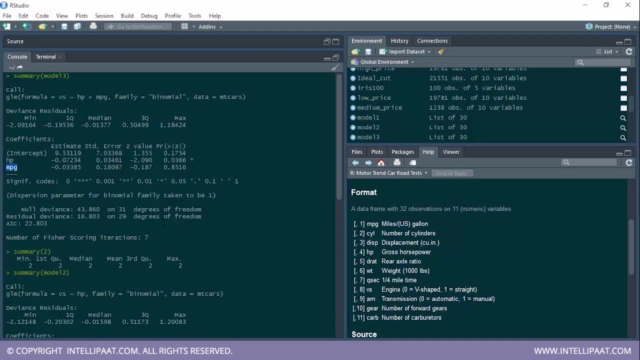 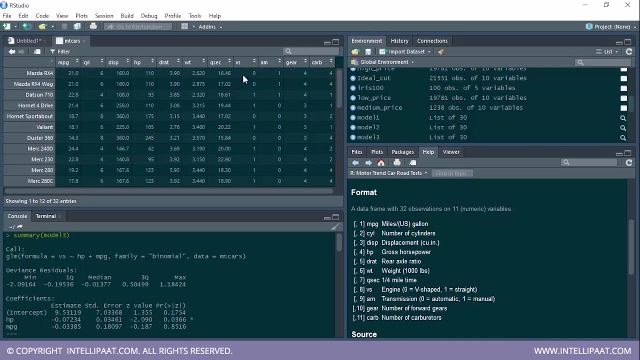 just deteriorating the accuracy of the model. thus we can basically conclude from all three of these is that model 2 is the best fit model. or, in other terms, if we want to determine whether the car has a v-type engine or an V-type engine or an AIC engine, then we can conclude that model 2 is the best fit model. or, in other terms, if we want to determine whether the car has a v-type engine or an 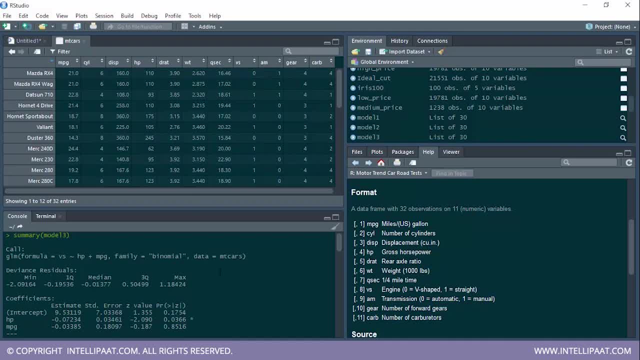 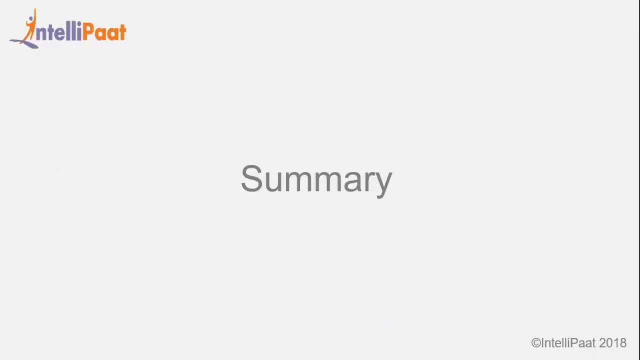 S-type engine, then it would be better to use HP as the independent variable, right? so this is how we can implement logistic regression in R right now, and this brings us to the end of the video. so let's have a brief recap of what we went through. so we started off. 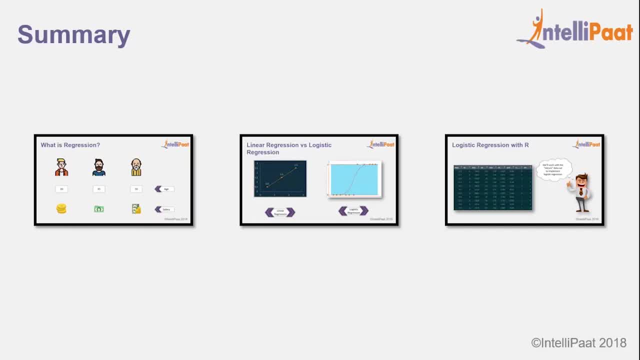 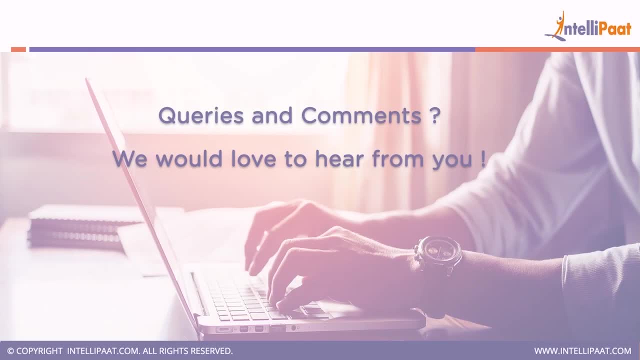 by understanding what exactly is regression, then we understood what is logistic regression and finally, we implemented the concept of logistic regression in R. Thank you for watching our video. Do like and share it. If you have any questions, comment below and we'll respond to them as soon as possible. 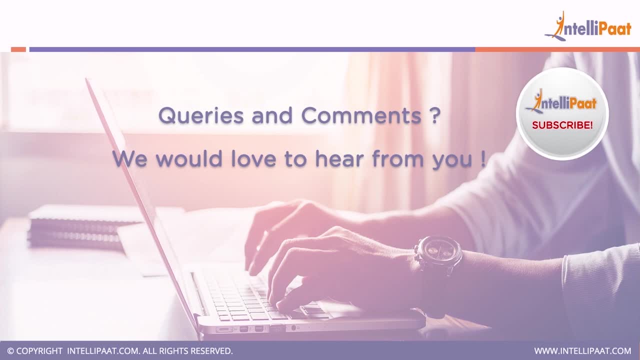 Also, do subscribe to Intellipaat channel so that you can keep yourself updated on the latest technologies. You can also go through other related videos in our playlist And, for more information, visit our website. Keep learning, keep improving.